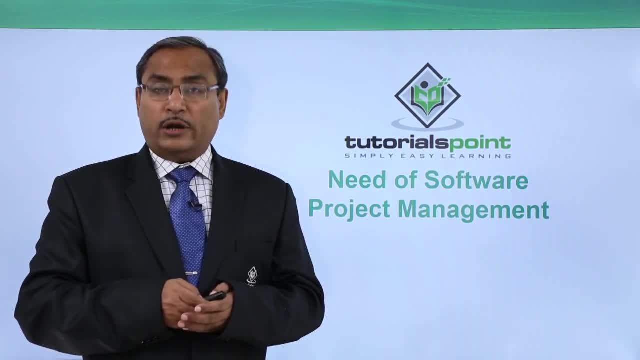 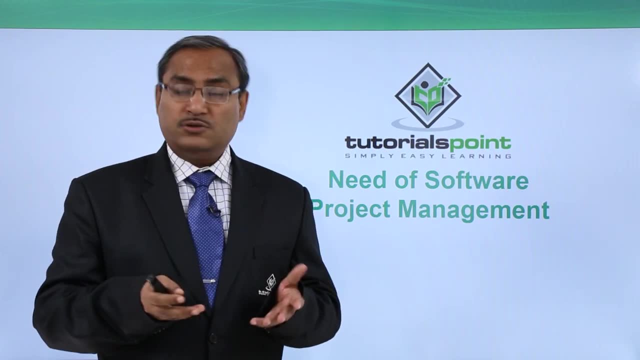 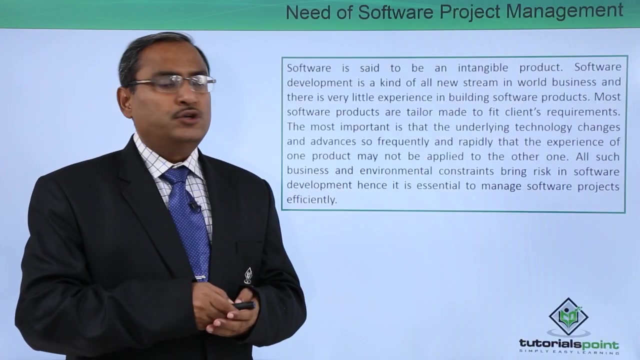 that we can check whether the project progress is in accordance with whatever we planned earlier. So that is why a project with project management may or may not fail. So that is very striking one. So now let us go for the software project management and need of software project management. 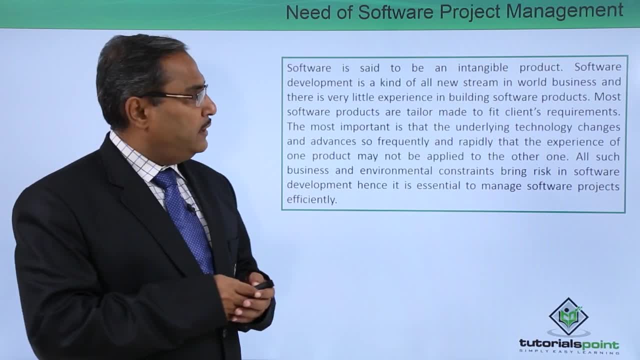 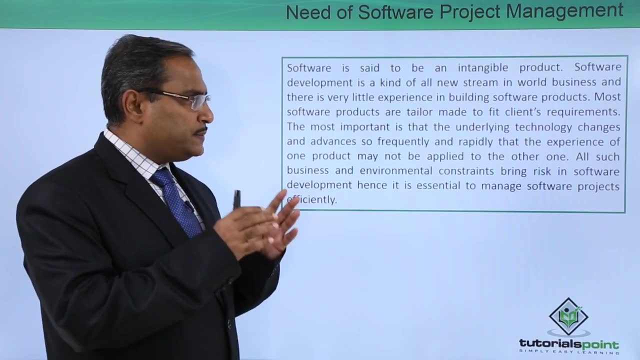 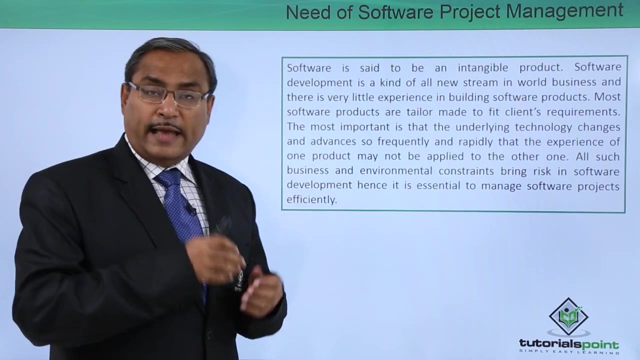 Software is said to be an intangible product You cannot touch and feel, And software development is a kind of all new stream in world business and there is very little, There is very little experience in building software products And most software products are tailor made to fit the clients requirements and according. 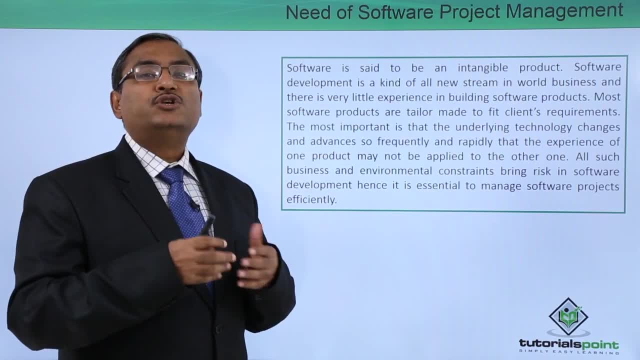 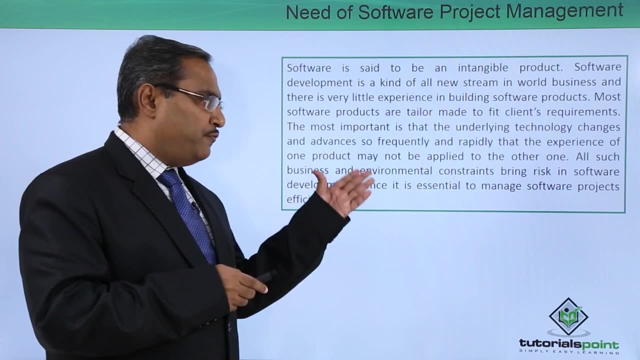 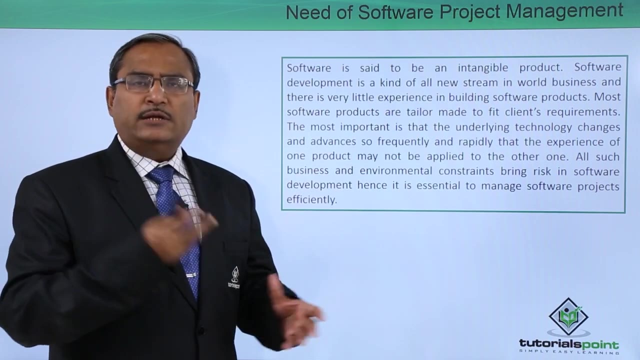 to the clients requirements, we are supposed to develop the software. The most important is that the underlying technology changes and advances so frequently and rapidly that the experience of one product may not be applied to other one. The technology is changing very rapidly, So as a result of that, 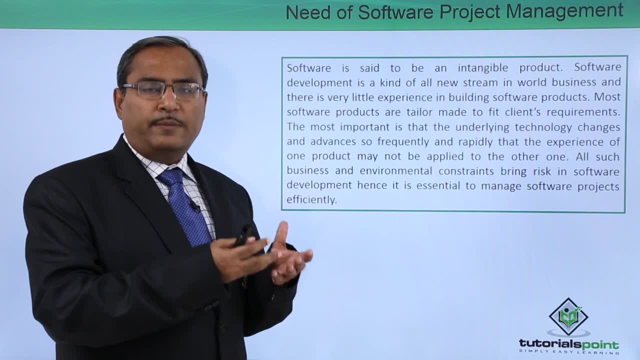 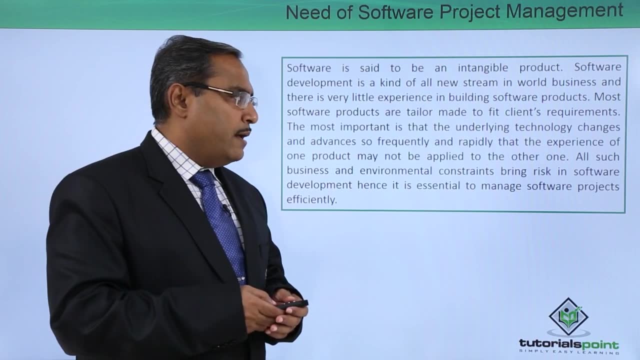 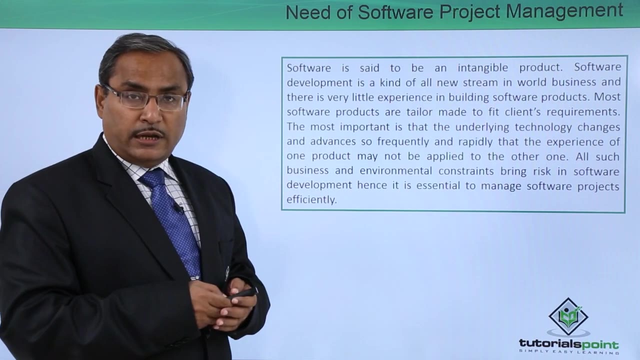 Whatever the experience we gathered from one technology based software development may not be applied on to the other. So all such business and environmental constraints bring risk in software development. hence it is essential to manage software projects efficiently, with the proper monitoring and control and with the proper project management. 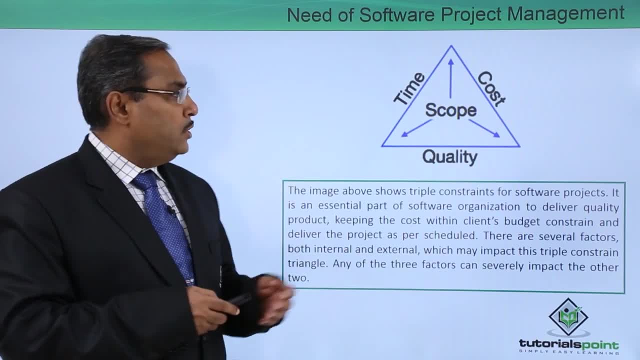 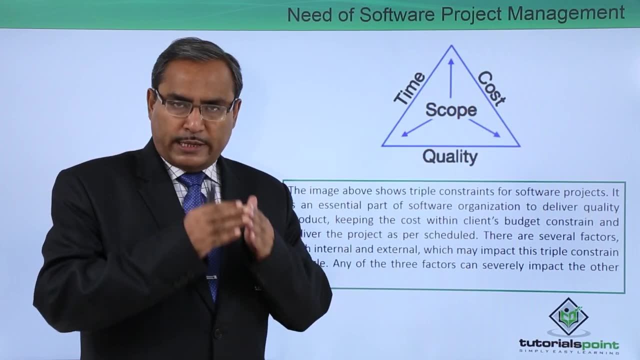 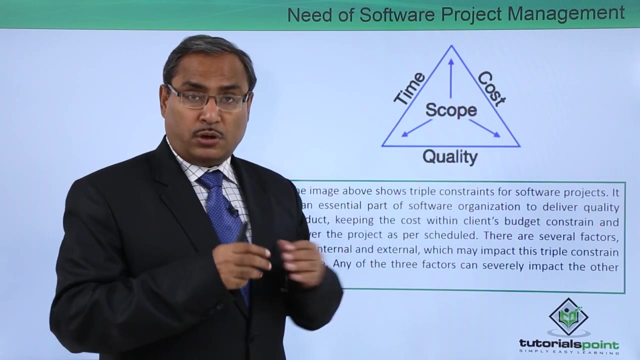 So now here we are considering the triple constraint theorem. So here we are having this time Where the price is used, the cost and quality. We are suppose to develop the project within the time frame. So that is a time constraint. We are suppose to develop the project within the budget. 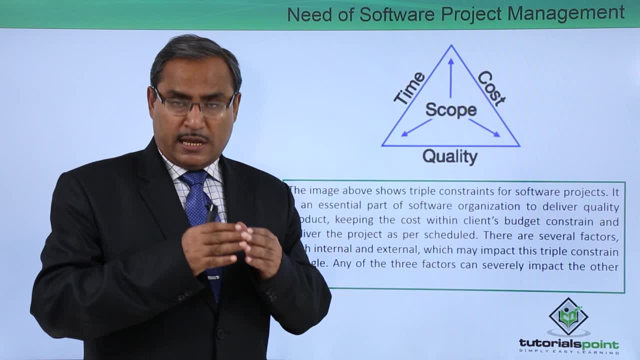 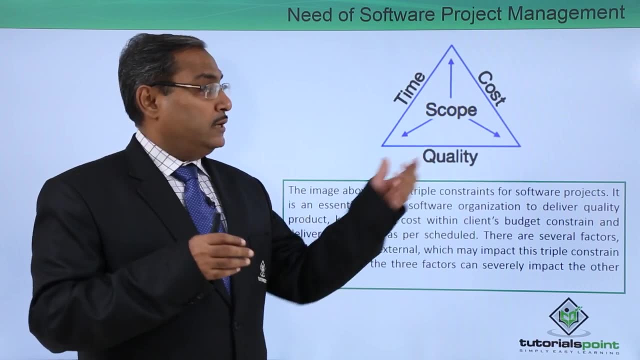 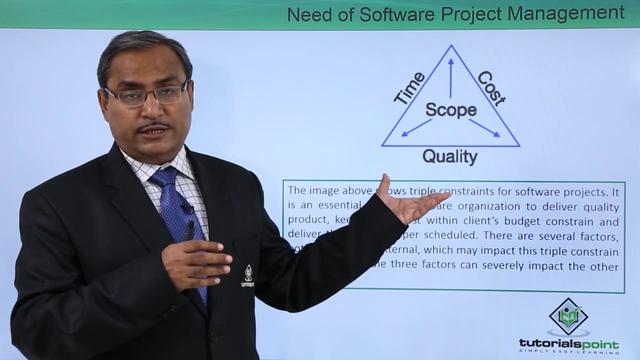 That is the cost constraint And we are suppose to implement all the features in according to the clients requirement and expectation. So that is a quality of the project. So that means the quality of the project means whatever we gathered at the earlier stage must have got implemented. the software should. 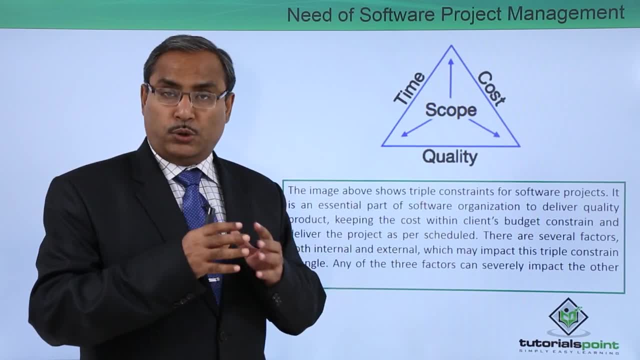 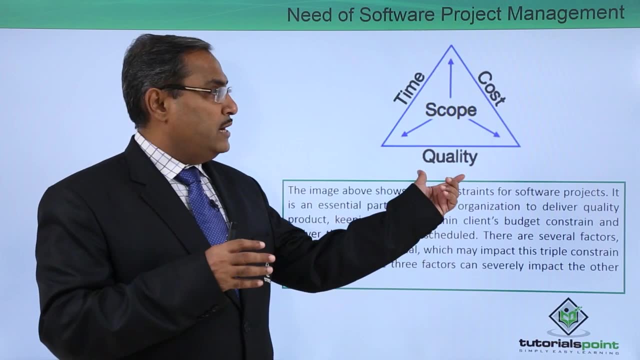 be reliable. the software should be safe. the software should be secured. the software should be user friendly. the software should be well, well versed with the current technology. so that is the quality. so there is a time, there is a deadline, there is a cost, there is a budget.